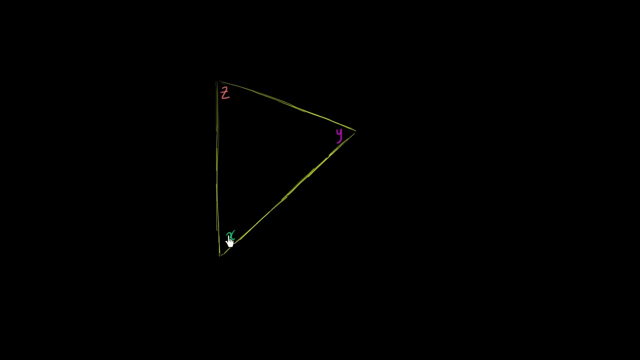 I've drawn an arbitrary triangle right over here And I've labeled the measures of the interior angles. The measure of this angle is x, this one's y, this one is z, And what I want to prove is that the sum of the measures of the interior angles of a triangle 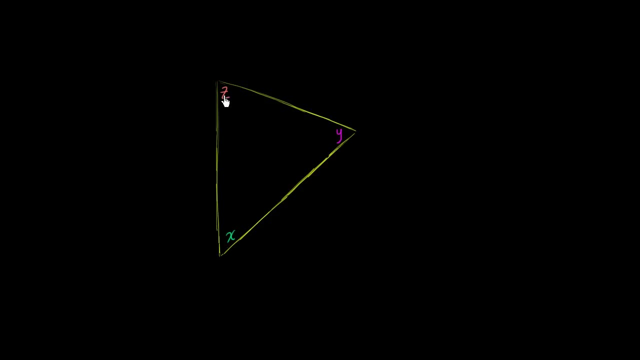 that x plus y plus z is equal to 180 degrees. And the way that I'm going to do it is using our knowledge of parallel lines, or transversals of parallel lines and corresponding angles. And to do that, I'm going to extend. 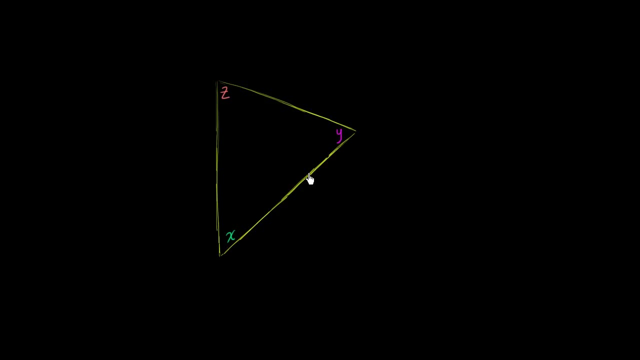 each of these sides of the triangle, which right now are line segments but extend them into lines, So this side down here. if I keep going on and on forever in the same directions, then now all of a sudden, I have an orange line. 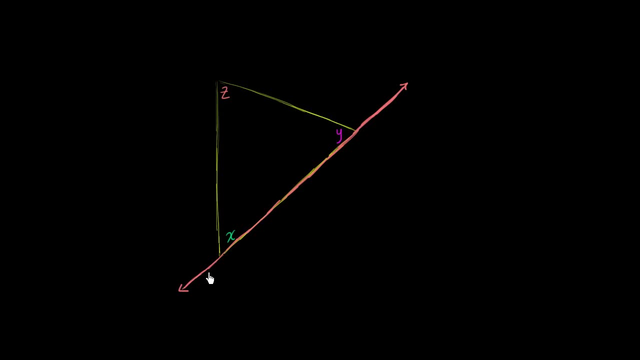 And what I want to do is construct another line that is parallel to the orange line that goes through this vertex of the triangle right over here, And I can always do that. I can just start from this point and go in the same direction as this line, and I will never intersect. 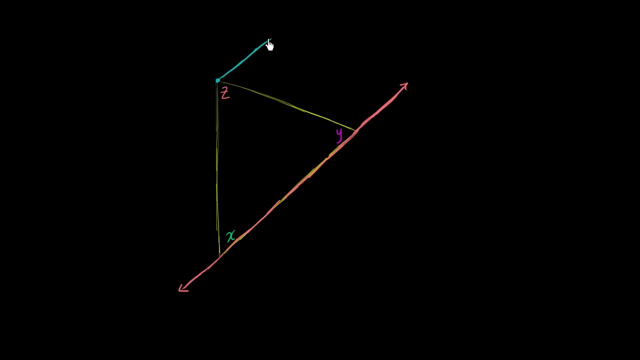 I'm not getting any closer or further away from that line, So I'm never going to intersect. I'm never going to intersect that line. So these two lines right over here are parallel. This is parallel to that. Now I'm going to go to the other two sides. 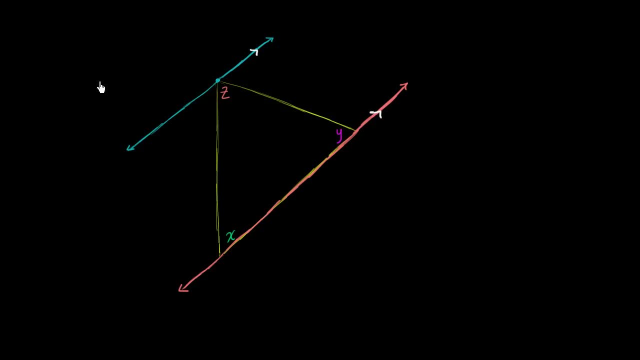 of my original triangle and extend them into lines. So I'm going to extend this one into a line. So there we go. I'll do that as neatly as I can. So I'm going to extend that into a line And you see that this is clearly a transversal. 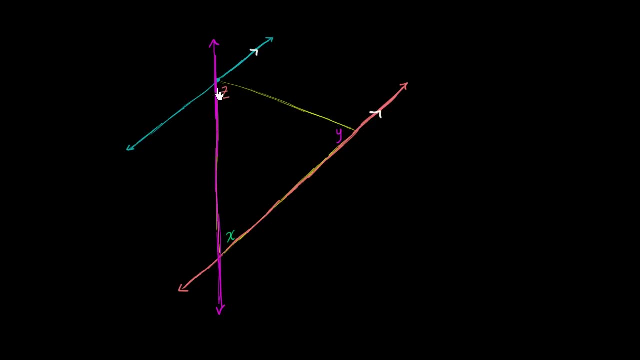 of these two parallel lines. Now, if we have a transversal here of two parallel lines, then we must have some corresponding angles. And we see that this angle is formed when the transversal intersects the bottom orange line. Well, what's the corresponding angle? 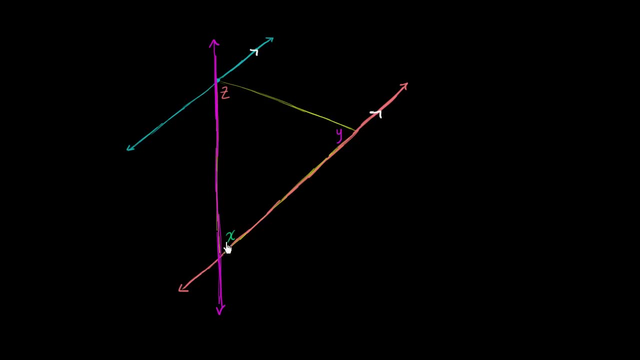 when the transversal intersects this top blue line, What's the angle on the top right of the intersection? The angle on the top right of the intersection must also be x. The other thing that pops out at you is: there's another vertical angle with x. 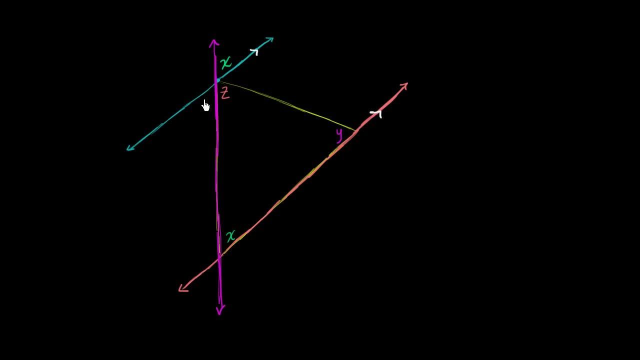 another angle that must be equivalent On the opposite side of this intersection. you have this angle right over here. These two angles are vertical, So if this has measure x, then this one must have measure x as well. Let's do the same thing with the last side of the triangle. 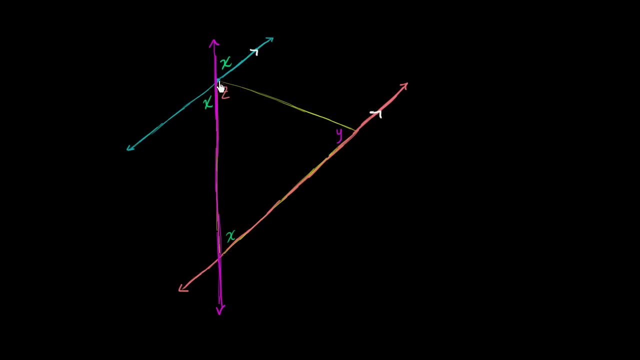 that we have not extended into a line yet. So let's do that. So if we take this one, so we just keep going, So it becomes a line. So now it becomes a transversal of the two parallel lines, just like the magenta line did. 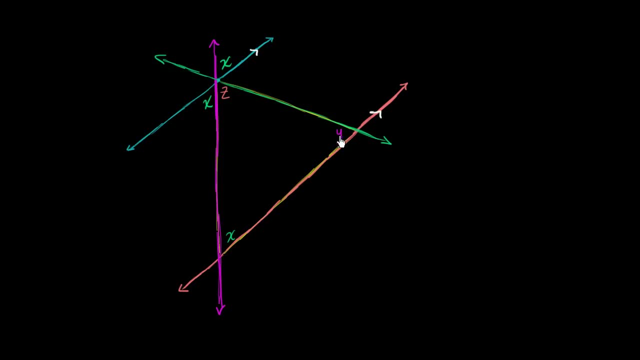 And we say: hey look, this angle y right over here. this angle is formed from the intersection of the transversal and the bottom parallel line. What angle does it correspond to up here? Well, this is kind of on the left side of the intersection. 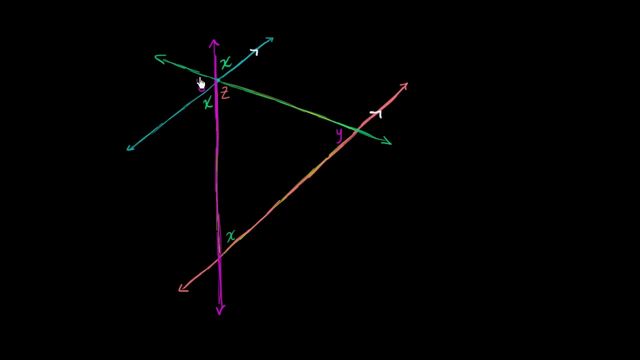 It corresponds to this angle right over here, where the green line, the green transversal, intersects the blue parallel line. Well, what angle is vertical to it? Well, this angle, So this is going to have angle, or it's. 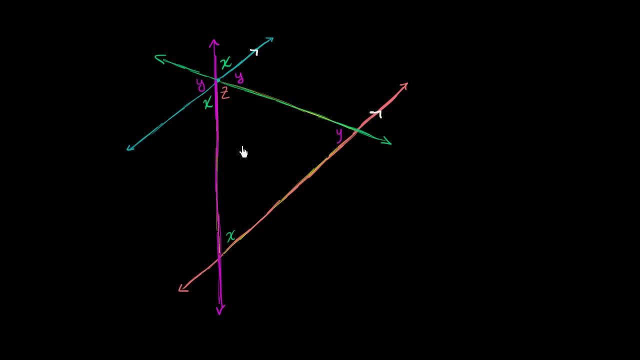 going to measure y as well. So now we're really at the home stretch of our proof, Because we will see that the measure we have this angle and this angle, This has measure angle x, This has measure z. They're both adjacent angles. 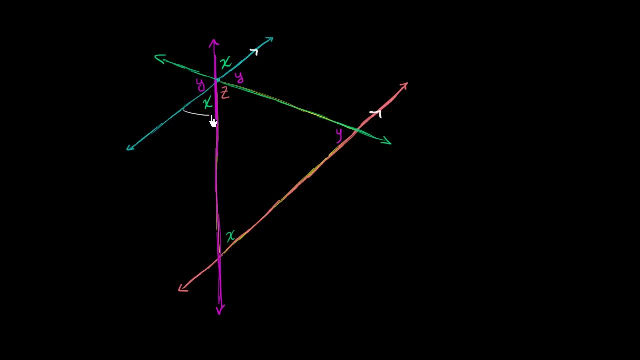 If we take the two outer rays that form the angle and we think about this angle right over here, what's this measure of this wide angle right over there? Well, it's going to be x plus z, And that angle is supplementary to this angle right over here. 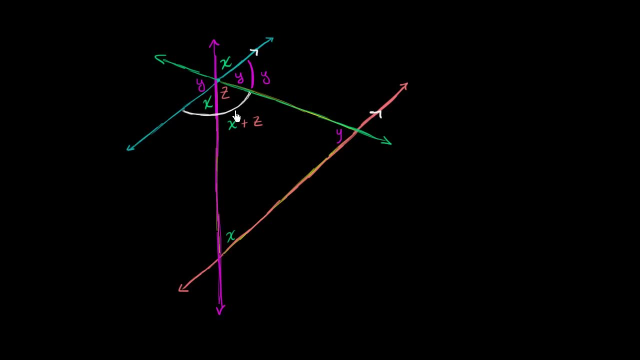 that has measure y. So the measure of this wide angle, which is x plus z, plus the measure of this magenta angle, which is y, must be equal to 180 degrees, Because these two angles are supplementary, So x. so the measure of the wide angle, x plus z. 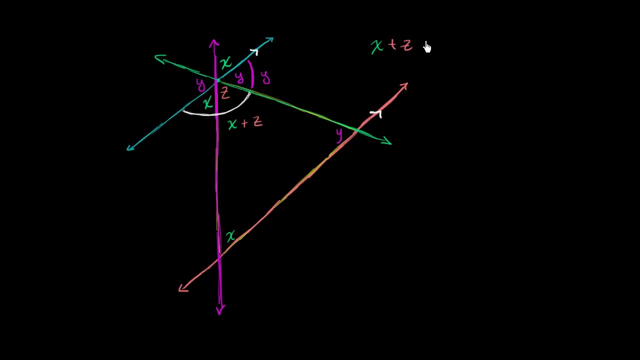 plus the measure of the magenta angle, which is supplementary to the wide angle. it must be equal to 180 degrees Because they are supplementary. Well, we could just reorder this if we want to put it in alphabetical order, But we've just completed our proof. 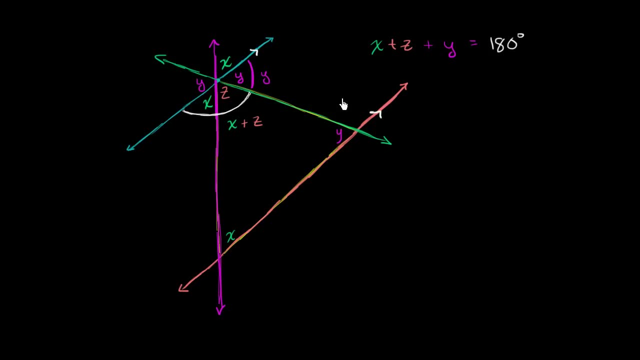 The measure of the interior angles of the triangle: x plus z plus y. We could write this as x plus y plus z. if the lack of alphabetical order is making you uncomfortable, We could just rewrite this as: x plus y plus z is equal to 180.. 180 degrees And we are done. 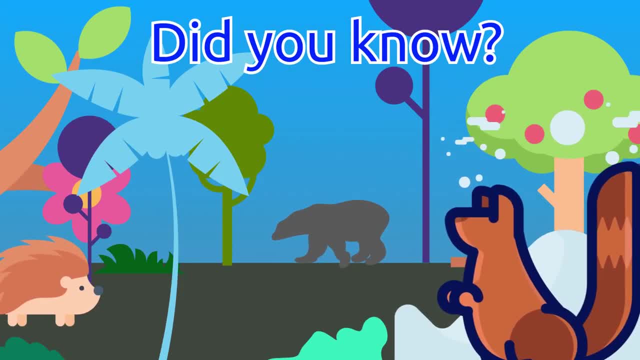 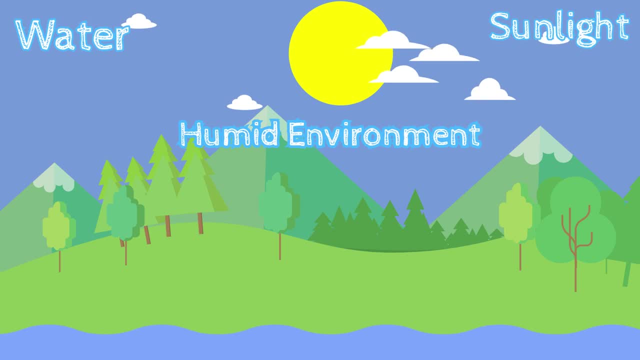 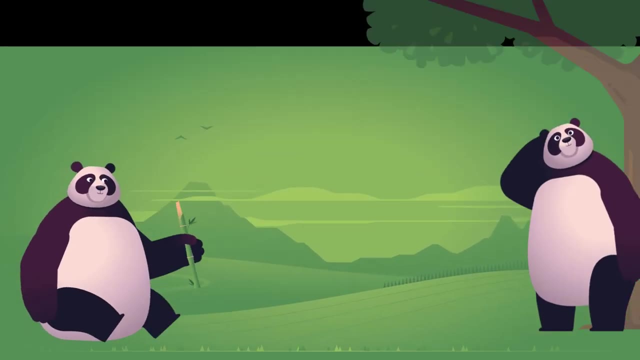 Did you know that up to half of the world's species all live in tropical rainforests? Water, sunlight and a humid environment are some of the factors that create the perfect living conditions for millions of species of plants and animals to thrive. Biologists use. 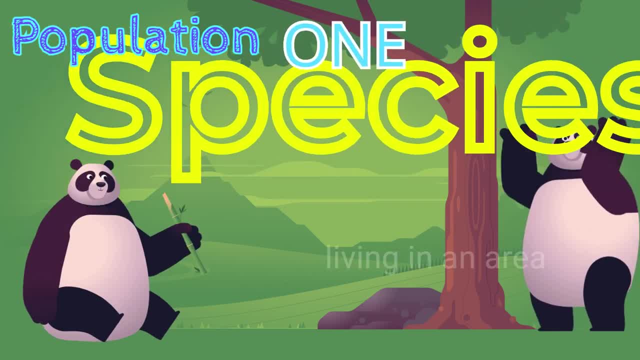 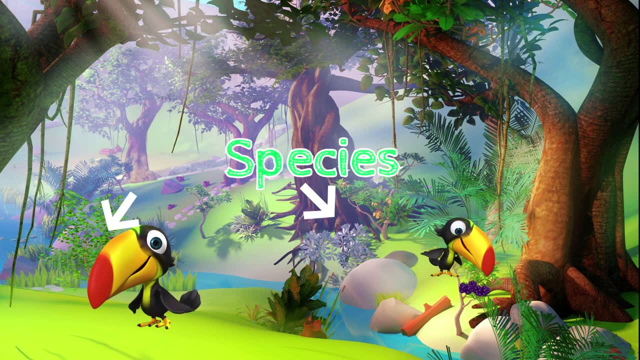 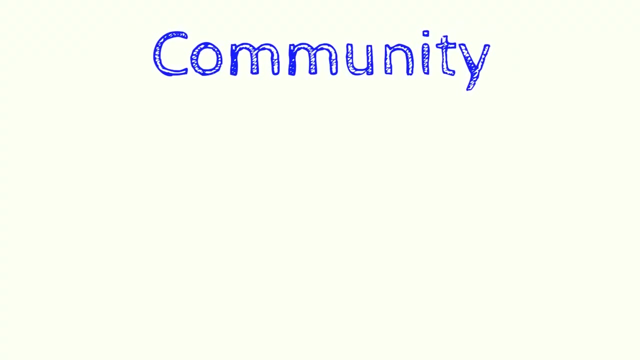 the term population to define all members of one species living in an area. For example, the toucan is the species of bird that is most populous in the Amazon. This is an example of a population. Biologists use the word community to define two or more species. 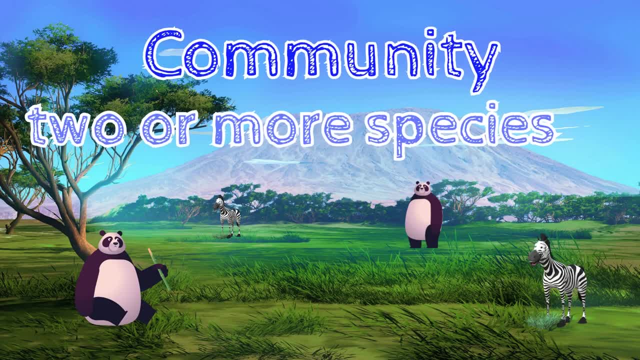 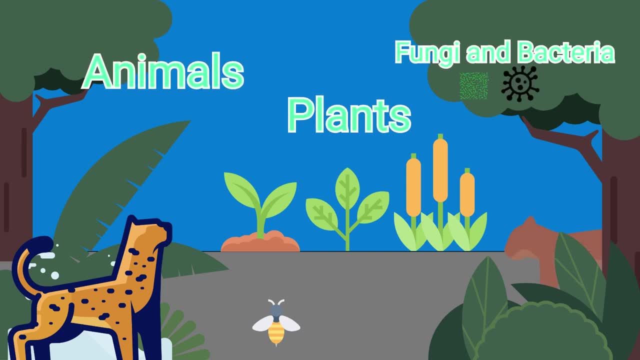 that interact with each other in a particular area. In a rainforest, various species of plants, animals, fungi and bacteria depend on each other to survive. An ecosystem is a community of species that really blend together. untilessaole and araucaria conquer between species. 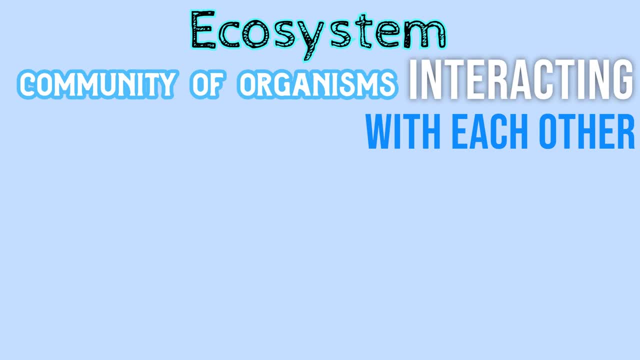 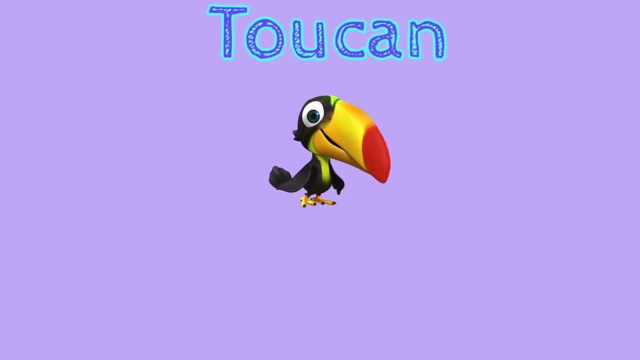 An ecosystem is a community of species that really blend together. untilessaole and araucaria conquer between species. An ecosystem is a community of of organisms interacting with each other, but also with the non-living components of their environment. For example, the toucan bird needs water, oxygen, humidity. 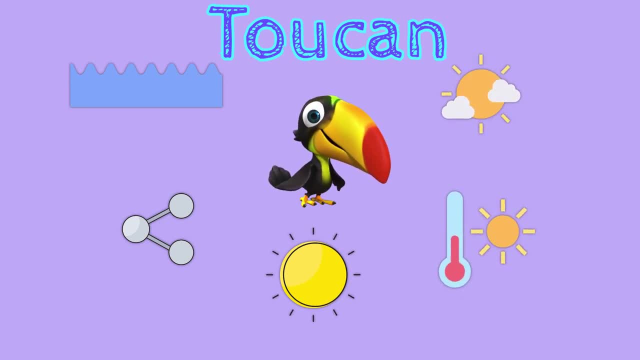 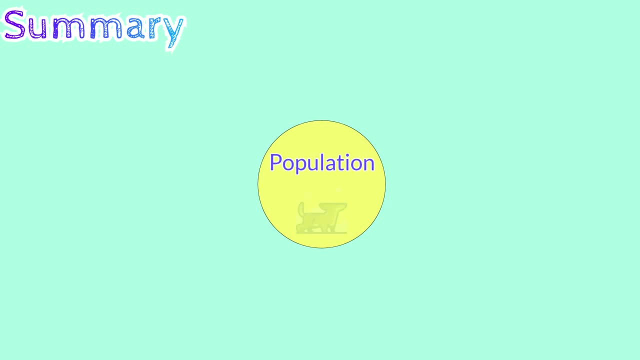 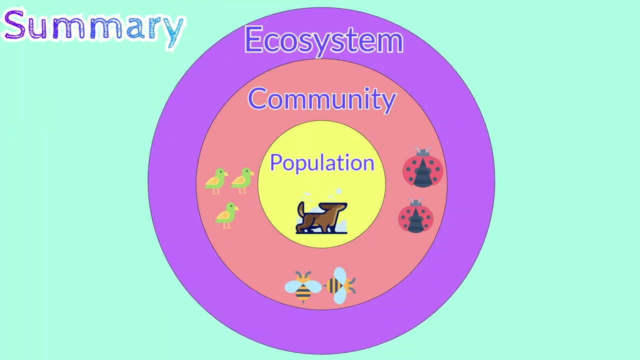 warm temperature and sunlight to survive. These are all non-living components. In summary, a population refers to one species. A community is made up of two or more species. An ecosystem is defined as all living organisms and their interactions with an environment. 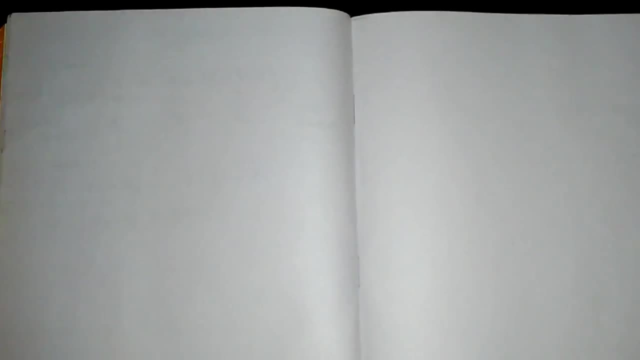 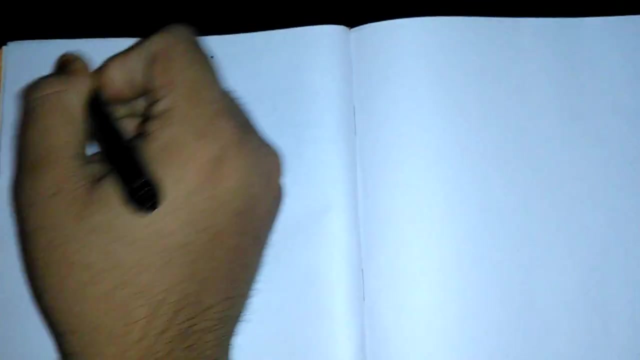 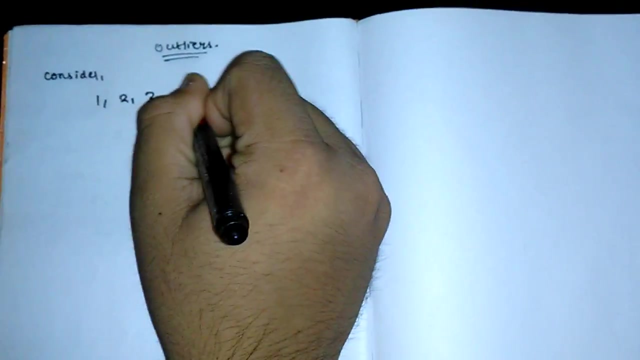 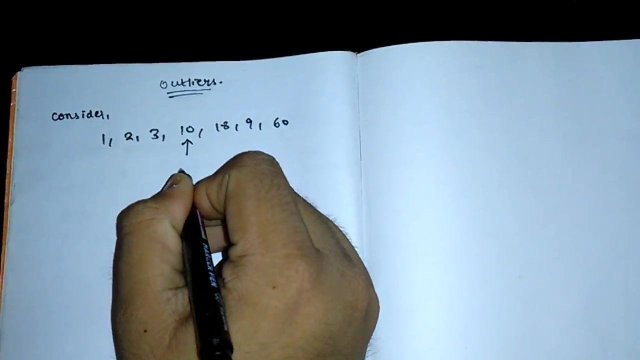 In this video we will try to learn about how to detect an outlier from a given sequence and how to plot it in a box plot. First of all, consider a given sequence: 1, 2, 3, 10, 18, 9, 60. now, as for the previous video, 10 is the median value.